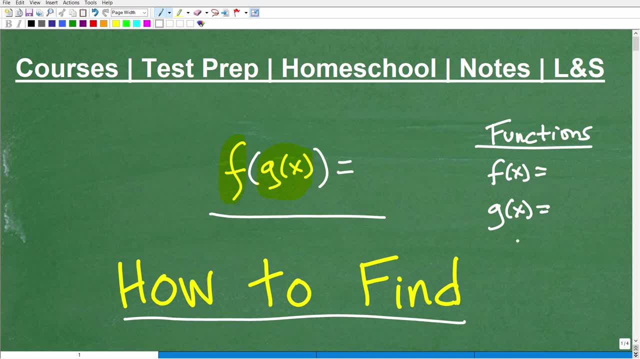 I have actual functions here that we're going to use as an example to cover what we're talking about, which, of course, is composite functions. When you have two or more functions, you can do all sorts of things, all sorts of function. 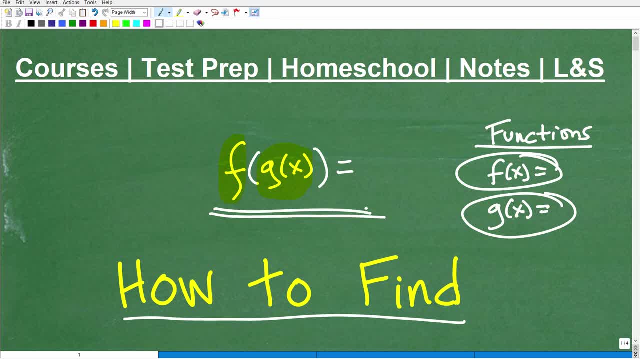 operations. You can add, subtract, multiply and, of course, do this, which is called a composite function. This seems to confuse a lot of students who are taking algebra. So if you are struggling a bit with composite functions, you're not alone, But let's go ahead and make it very easy for you. 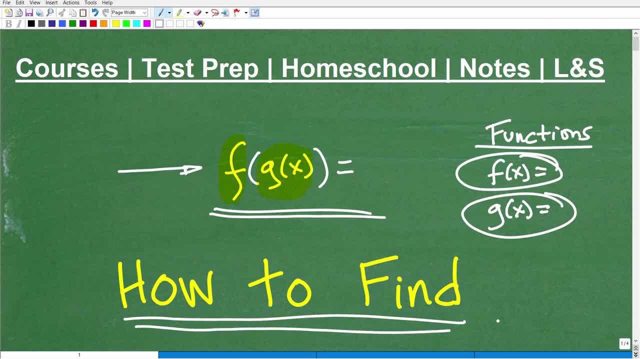 to understand this, and that's going to be the objective of this little video. But before we get going, let me go ahead and quickly introduce myself. My name is Algebra 1, and I'm going to introduce myself. My name is John. I'm the founder of TC Math Academy. I'm also a middle and high. 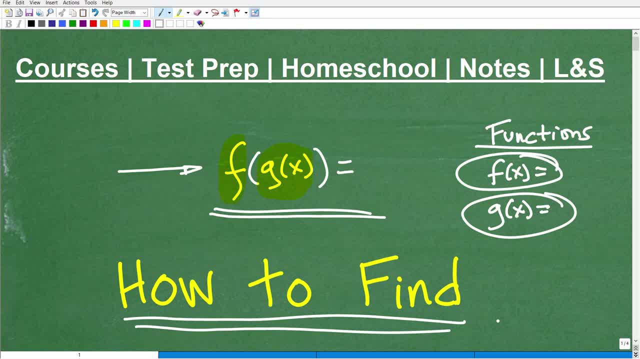 school math teacher. I've been teaching math for decades And if you're struggling in math, I'm telling you right now: don't give up. What you need to be successful in math is great math instruction- clear, understandable and comprehensive. So you need more than just quick, little. 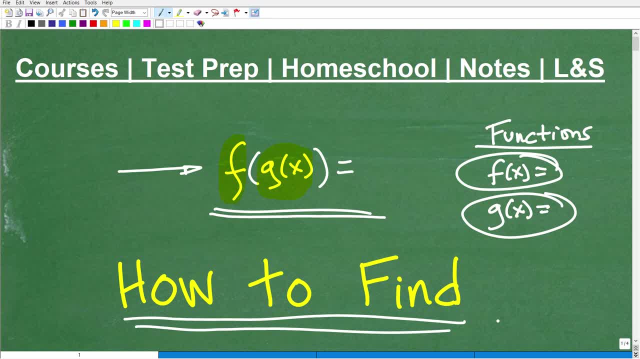 YouTube videos or short tutorials. You need full instruction and that's where I can help you out. So if you're at the middle school, high school or college level, check out my math help program. You can find a link to it. 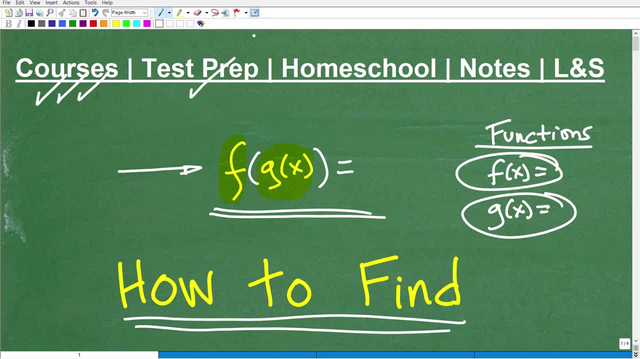 In the description of this video. I promise you it will help you out. Also, if you happen to be preparing for some sort of test with the math section- things like the SAT, ACT, GED, ASVAB, maybe a teacher certification exam- I have a ton of test prep courses that can help you out Also. 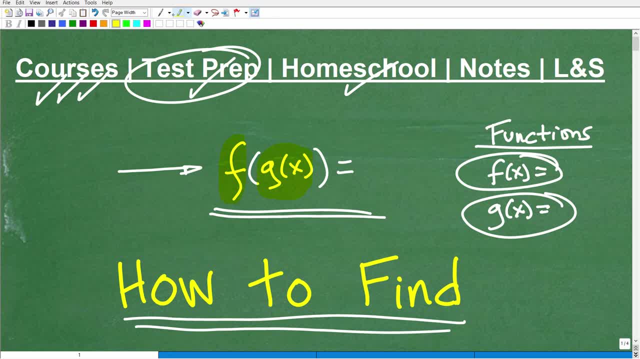 if you're a homeschooler, I have excellent middle and high school math courses that you might want to explore. By the way, if you need a pair of math notes, if your notes aren't up to speed- and this is a common weak area for those of you that are struggling to math- I'm going to leave. 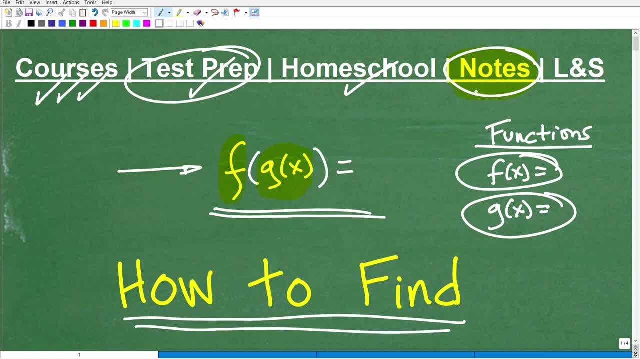 a link or links to my math course. So if you're a middle or high school math teacher, I'm going to leave a link to my notes- various notes- in the description of this video as well. And if this little video helps you out, don't forget to like and subscribe, as that helps me. 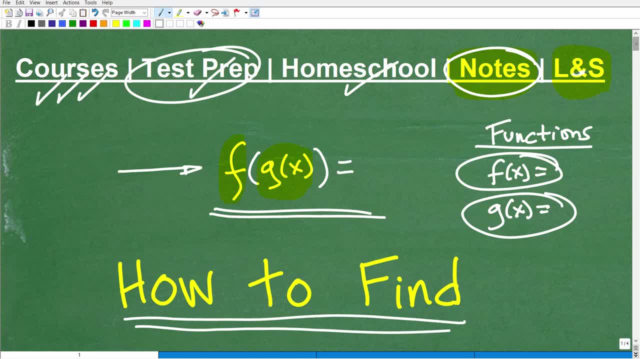 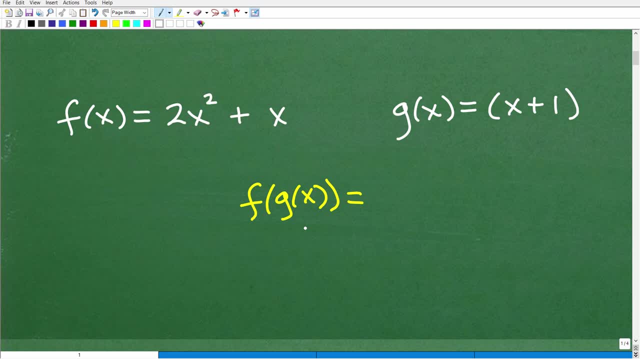 out big time. Okay, so let's get into composite functions, And again we need some actual functions to do a problem. So let's go ahead and take a look at this example here. So here I have an f function, an f of x function. This is just the name of a function, And here's my variable: x. 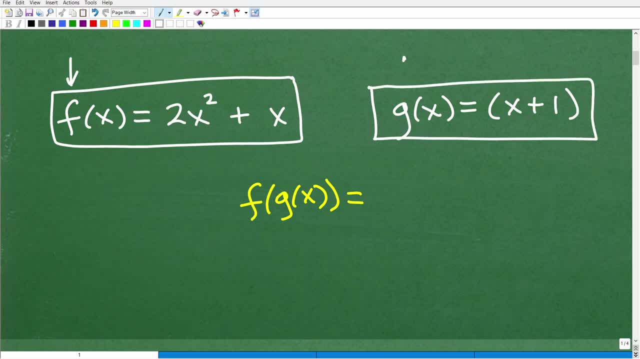 and I have another function over here. Its name is g. Okay, so this is the g of x function. So g of x is equal to x plus 1, and the f of x function is equal to 2x squared plus x. So you're asked to find f of g of x Again. 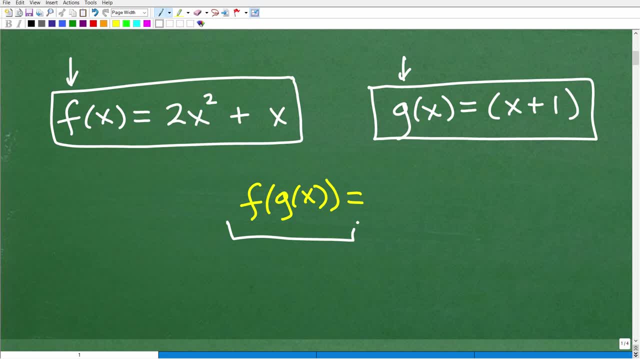 this is what we call a composite function. You absolutely need to know how to do this in algebra, And a lot of students get confused on this. They kind of do this. They're like, hmm, I always mess this up because this is, you know, confusing. Well, I'm telling you. 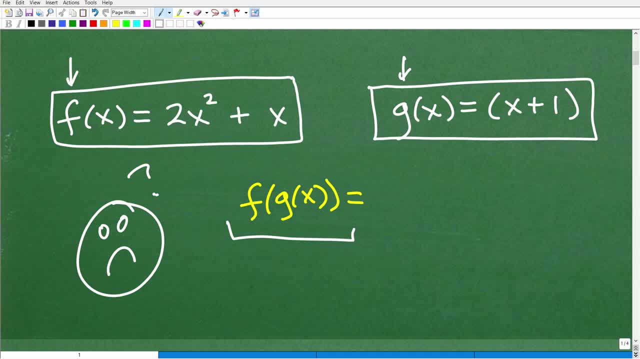 now it doesn't have to be confusing at all. Now I just kind of want to see where you're currently at. If you want to kind of check your current understanding of this, go ahead and compute f of g, of x or calculate this out. It'll probably take it about- oh, I don't know- 30. 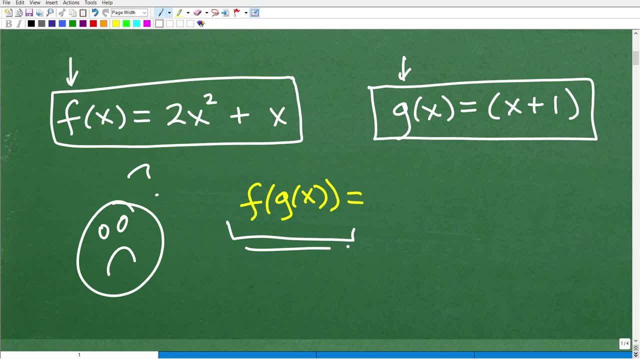 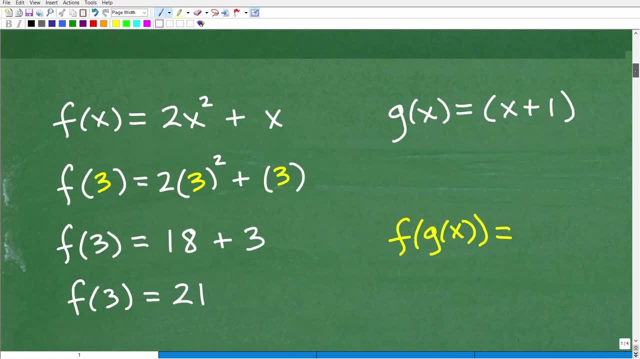 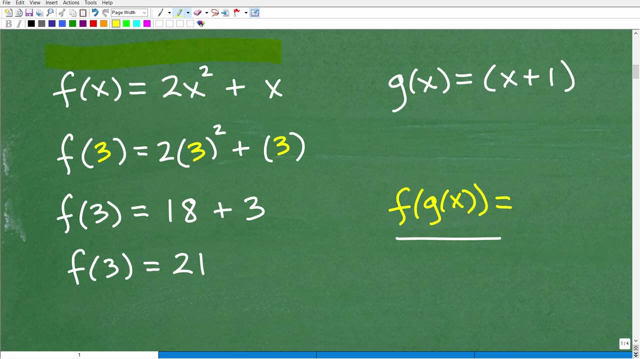 seconds to a minute. So if you want to pause the video and do that, I would suggest you go ahead and check your understanding. But I'm going to get into the solution now. Okay, so before we actually compute the composite function here, f of g of x. again, we have two functions here: the f function. 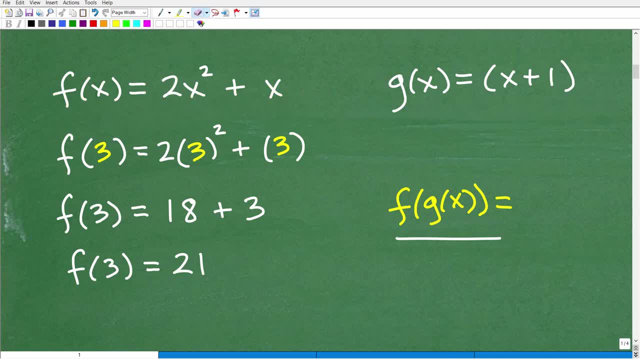 and the g function. Let's just talk about what we're doing big picture. Well, a composite function is basically we're evaluating the f function with the g function. But let's just review what it means just to evaluate a function with any particular value. So let's take the f of x. 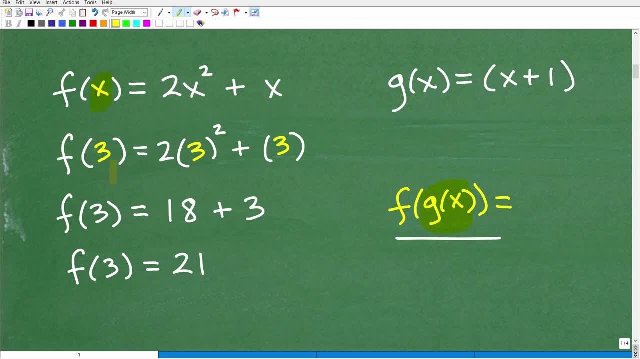 function here, If I wanted to find f of three. okay, So let's take the f of x function here. So let's say you're asked to find f of three. What does that mean? Well, it means that you're. 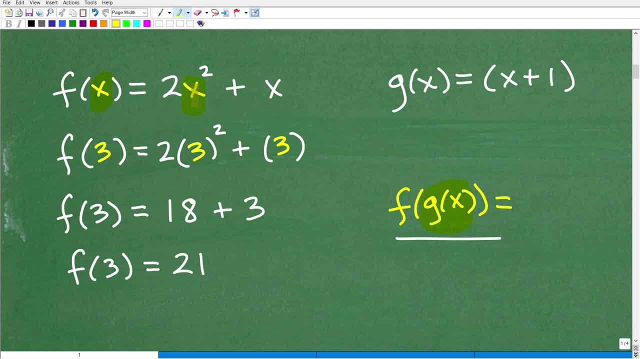 going to replace all the x's here, which, here is an x and here's an x. You're going to replace that x with the three. okay, Then we're going to go ahead and simplify. So, instead of 2x, squared. 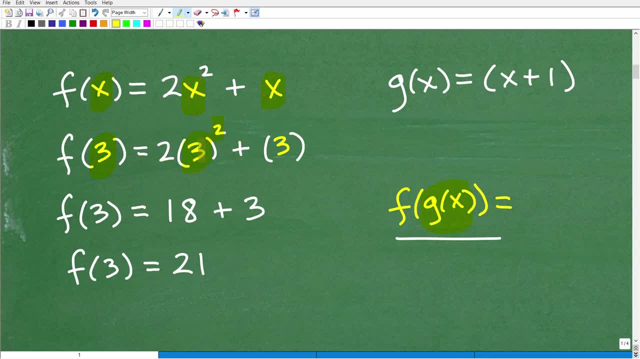 we're going to have 2, 3 squared plus, or 2 times 3 squared, excuse me- plus 3.. So we're replacing the variable x with the three, And now we're going to go ahead and just use our order of operations. 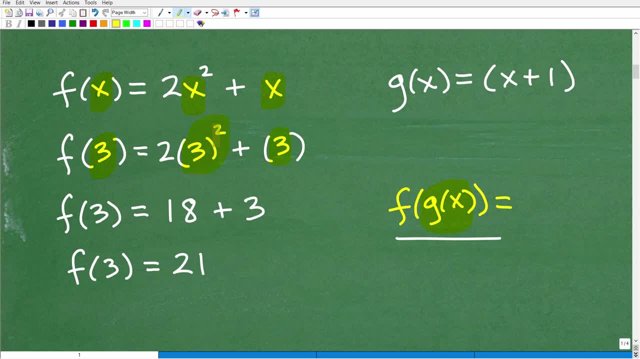 to simplify this Now we have 3, squared of course, is 9.. 9 times 2 is 18.. 18 plus this, 3 is 21.. So f of 3 is 21.. So before you can understand how to work with composite functions, 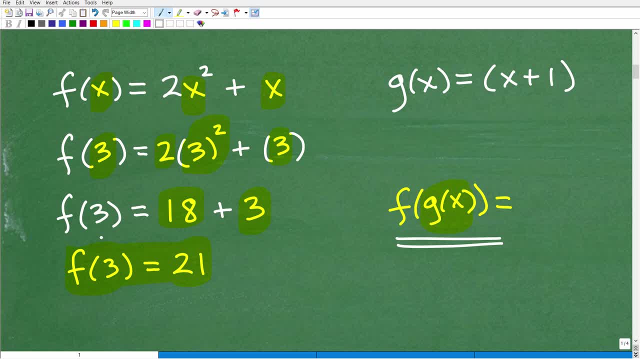 you need to obviously know how to evaluate a function, Because what we're doing here- f of g, of x- is, instead of plugging in a number- let me go ahead and write this a little better- instead of plugging in a number like 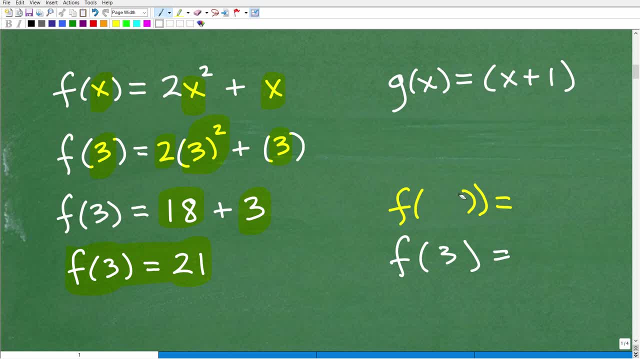 3 into the f function. I'm going to erase this so we can see this a little bit clearly, clearly, not clearly clearly. Okay, so what we're going to be doing, instead of plugging in 3 into the f function, we're going to be plugging in the g of x function. okay, But what does this? 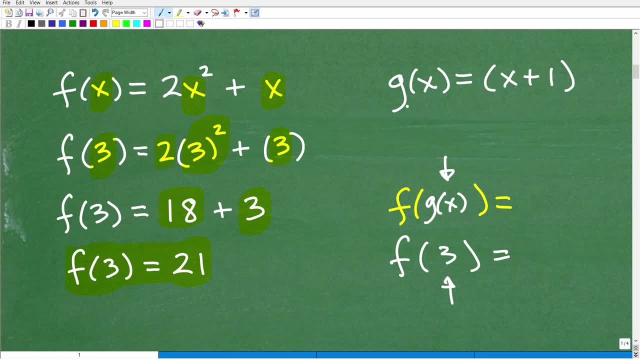 mean. This notation is confusing. Well, instead of this symbol here, g of x is the same thing as x plus 1, okay, So really, f of g of x is finding the function f of x plus 1, okay, What does that mean? Well, again, anytime you are. 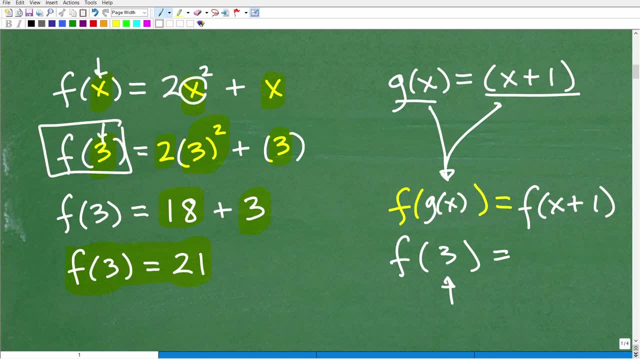 evaluating a function. whatever you plug in right here, you're going to replace these x's with whatever you plug in for what you're trying to evaluate. In this case, it's going to be x plus 1, and then we're going to simplify, okay, So let's go ahead and see how that works right now. 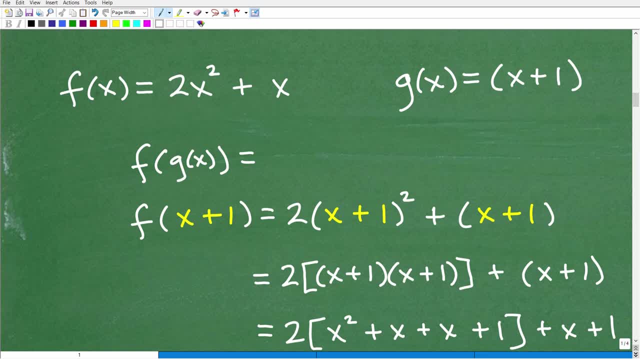 Okay, so here we go. So f of x is equal to 2x square plus x. g of x is equal to x plus 1, okay, Let's find f of g of x, meaning I'm going to plug. 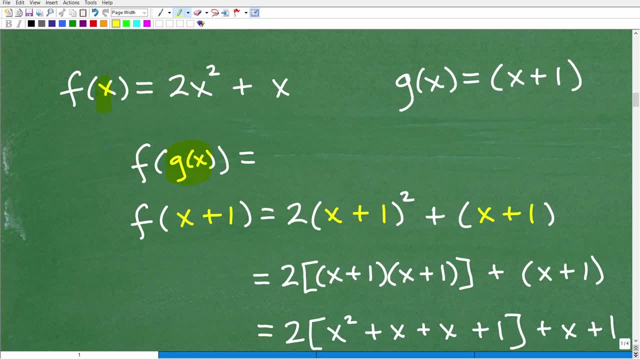 in the g of x function, okay, into the f function. So wherever I see an x, I'm going to replace it with the g of x. but that g of x I'm not going to use this thing, I'm going to use x plus 1,. 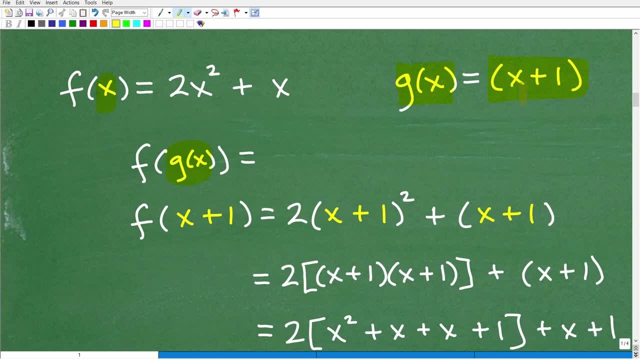 because x plus 1 is equal to g of x. So I'm using x plus 1, not g of x. So this x right here I'm going to replace with an x plus 1, and this I'm going to replace with an x plus 1.. So that's going to look like this, okay? F of g of x. 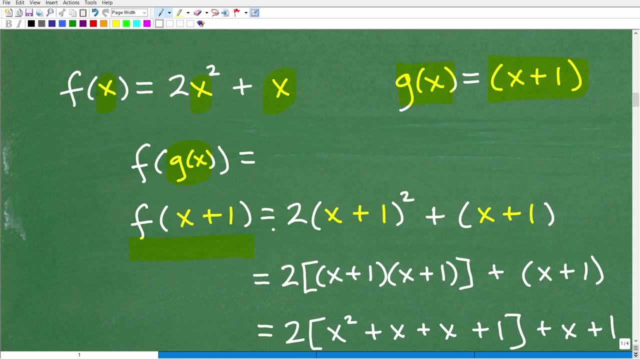 is effectively finding f of x plus 1.. So that's going to be equal to 2 times x plus 1 squared. okay, Again, right here, this x I'm replacing with x plus 1, and then I'm going to put a plus sign. 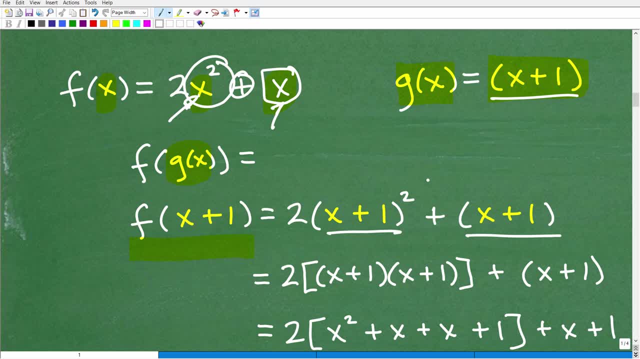 and then we have to add in another x plus 1.. So this here matches. okay, this setup up here, okay, All right. So the first most important thing when you're trying to figure out composite functions is just understanding the setup. So if you're like, okay, now I understand and really you wouldn't put f 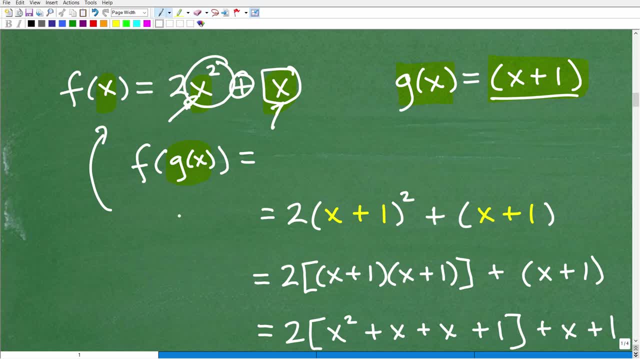 of x plus 1. there You would write, technically, you would write f of g of x, but I did that kind of to explicitly, you know, show you that g of x. what we're plugging in is x plus 1, because 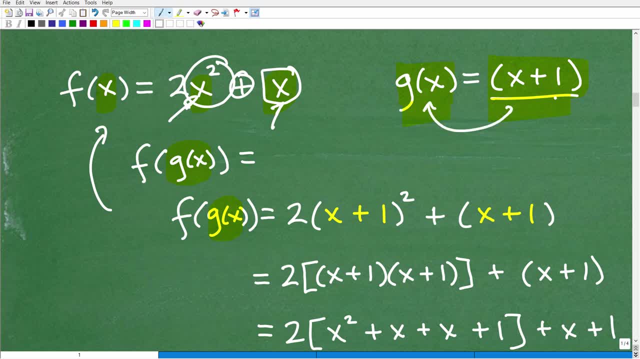 we're saying that g of x is equal to x plus 1.. So x plus 1 is the same thing as g of x. g of x is the same thing as g of x, So that's going to be equal to x plus 1, and then we're going to 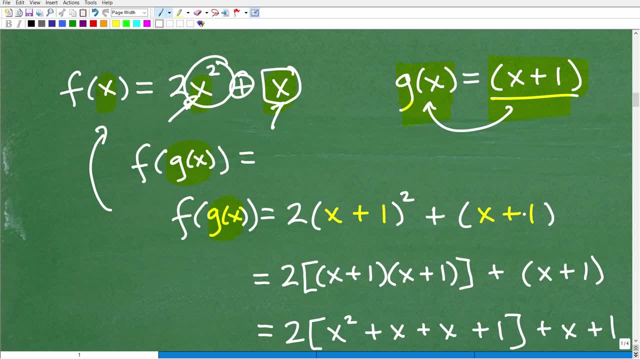 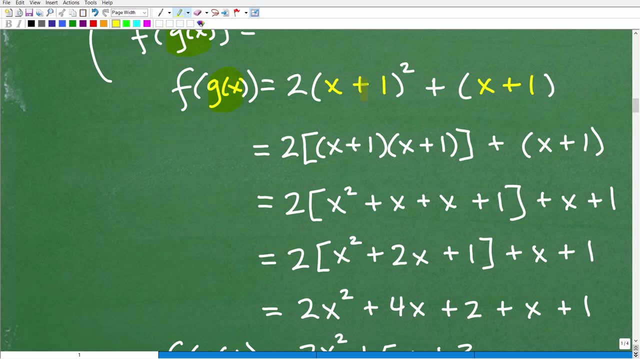 use x plus 1.. So this notation, this is how you would write this actually in your work. Okay, So at this point, what you have to do is use your awesome algebra skills to simplify this. So let's go ahead and do this now. So we have 2 times x plus 1 squared. 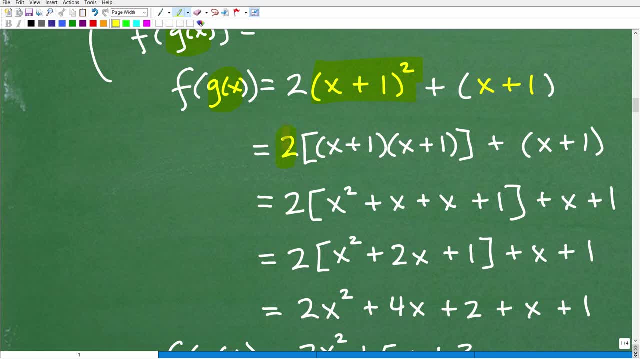 Of course we have to do powers before we do multiplication, So I would suggest using brackets. So just write it out this way: 2 times x plus 1, times x plus 1.. That means x plus 1 squared plus this x plus 1, right here, Okay? So always write it in your work. 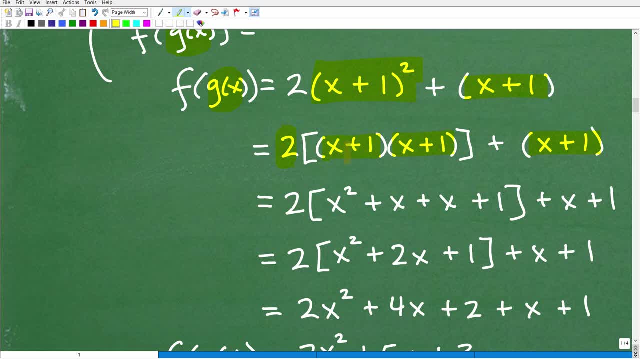 step by step, step by step. It will help you, you know, avoid making any errors. So let's go ahead and do this multiplication here: x plus 1 times x plus 1 is going to be x squared plus x plus x plus 1.. I'm just using a FOIL technique there. So we're going to multiply 2 by all of. 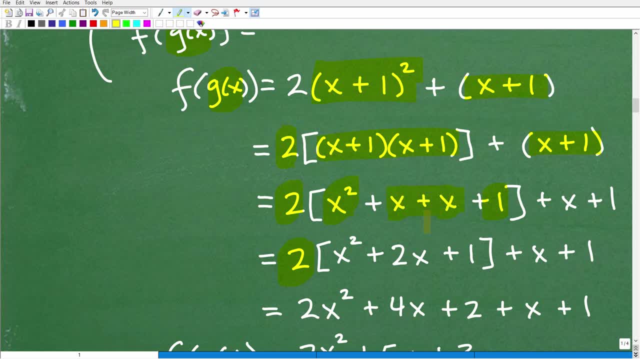 this. So let's go ahead and combine like terms. So this is x and x that's 2x. So we're going to have 2 times x squared plus 2x plus that 1.. And again, let's not forget this: x plus 1 over there. 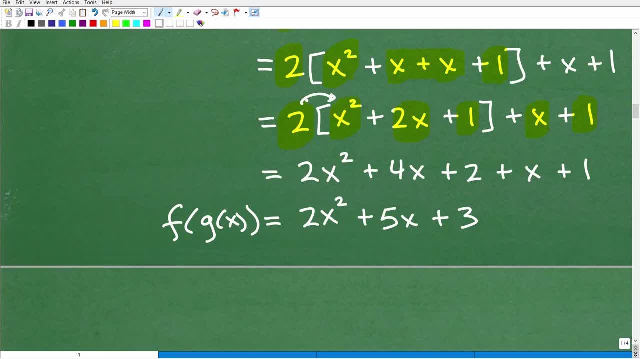 Okay. So now I'm going to go ahead and use the distributive property and multiply 2 by all this stuff inside the brackets. So 2 times x squared is 2x. squared 2 times 2x is 4x, And then 2 times. 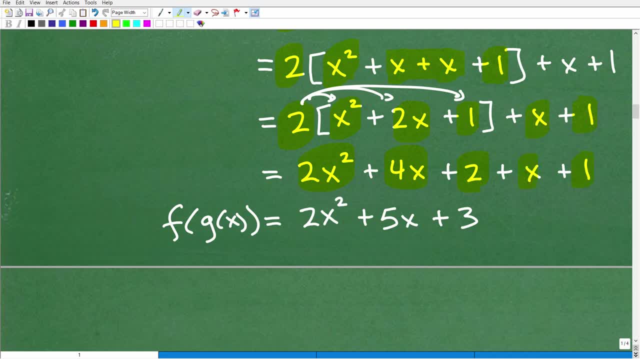 this 1 is 2 plus this x plus that 1.. Now I'm going to go ahead and combine like terms. Of course you're going to write this thing in standard form: highest to lowest power. So 2x squared. 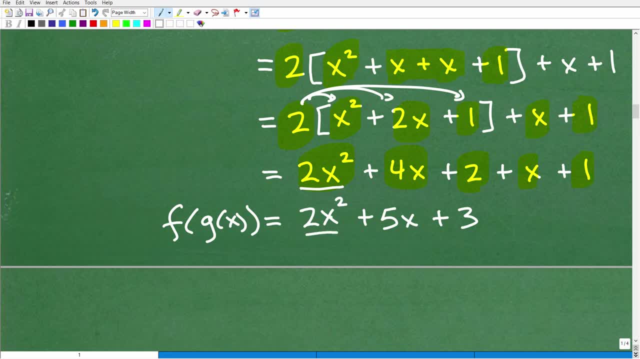 there is no other 2x, or there's no other x squared term. So our first term is going to be 2x squared, because it's the highest power of x. But we have a 4x and an x here, or 1x, So that will. 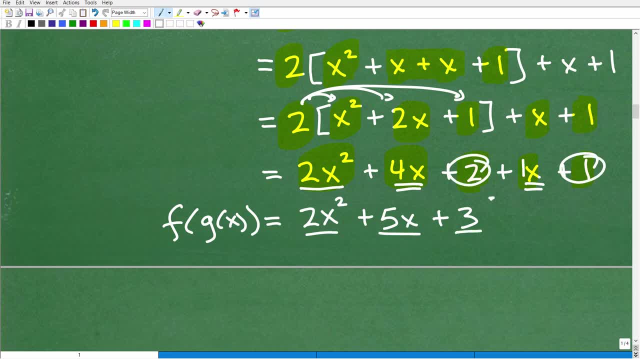 give us 5x, and then a 2 and a 1. that gives us 3.. So this is our final answer, right there. F of g of x is equal to 2x squared plus 5x plus 3.. Okay, How did you do? Did you get this right? And you? 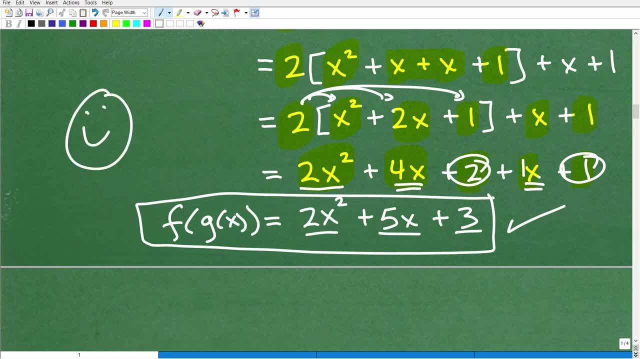 just kind of want to check your work. Well, if you got this right, I must go ahead and give you a lovely, happy face and a plus plus a 135 percent. Let me give you some extra stars here, just so you can have an awesome day. I will say that most. 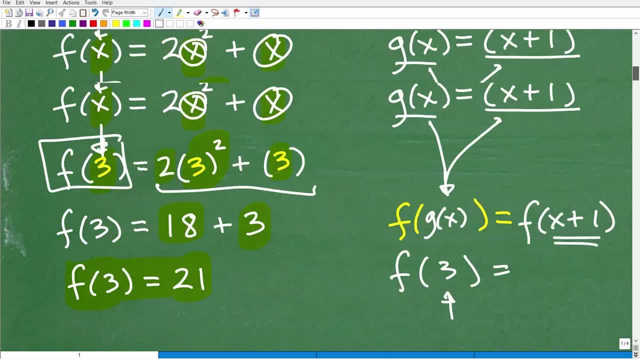 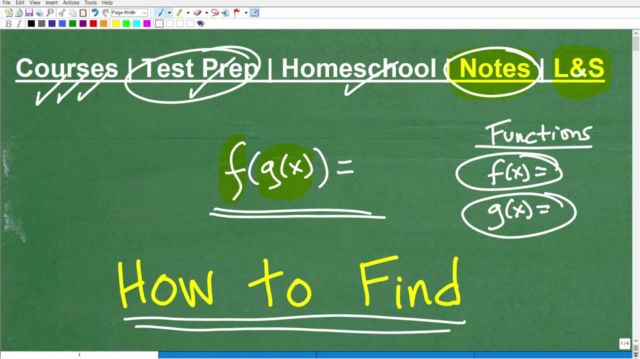 students get confused with composite functions when they're first learning about functions. Okay, So it's normal to you know struggle with this a bit, But I can tell you right now you're not going to avoid composite functions. Matter of fact, composite functions are everywhere in the 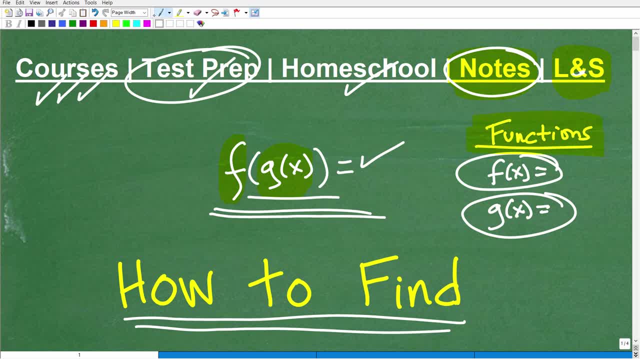 study of algebra. Okay, You're going to see it over and over, especially when you're dealing with topics like finding the inverse function. So you're just going to have to know how to work with functions. Again, function is a huge, huge topic And if you need additional help with functions, I'm going to 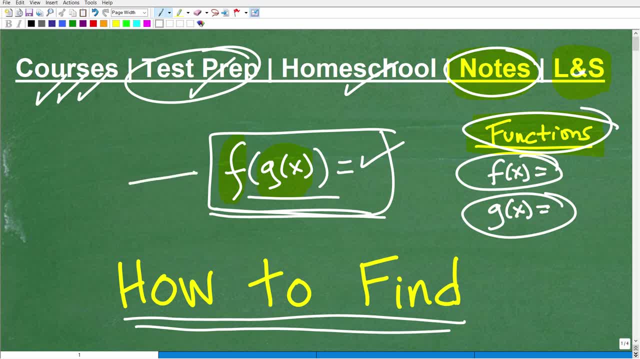 suggest a couple of things here. One, probably at this level you really get into this at the Algebra 1 level- and, of course, Algebra 2.. So I would definitely recommend my Algebra 1 and or Algebra 2 course, all depending on what level you're at My pre-algebra course you typically 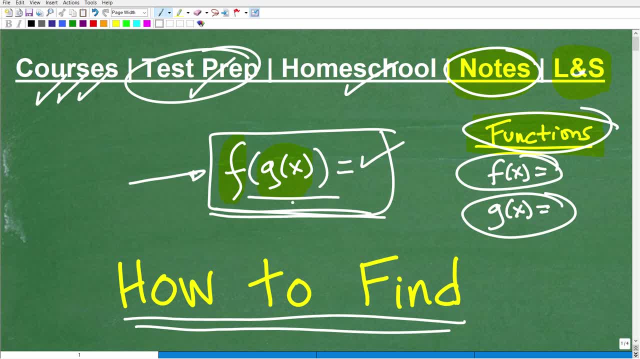 don't get into composite functions in pre-algebra, So I wouldn't suggest that, But I would suggest at least Algebra 1.. Also, I do have additional videos on my YouTube channel about functions. You can check that out as well, All right. So, with that being said, I definitely 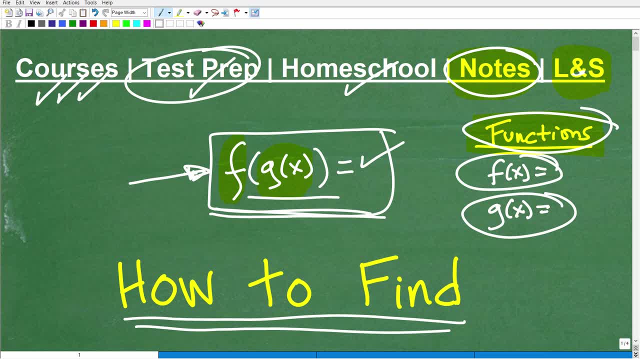 wish you all the best in your mathematics adventures. Thank you for your time and have a great day.